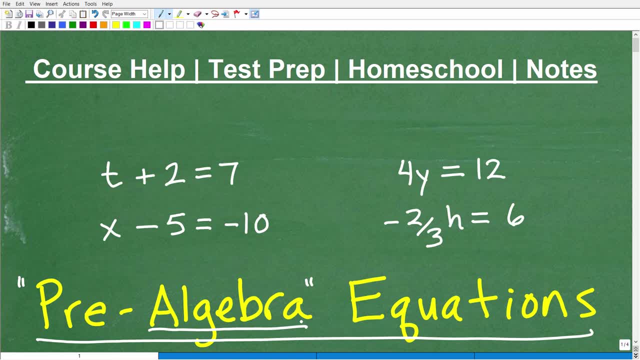 you're in fact learning algebra, Okay. so you're just not learning it at a complete, full level like an Algebra 1 course, so you're just kind of taking a lighter version of an algebra class, but indeed you are learning algebra. So if you think you know how to solve these four equations, go ahead. 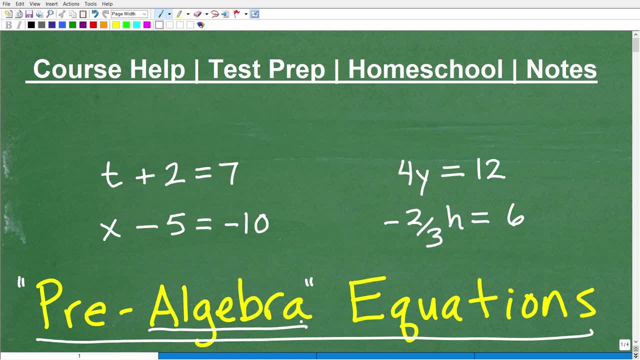 and pause the video and put your answers into the comment section. Of course, I'm going to solve these here in just one second, but first let me quickly introduce myself. My name is John. I'm the founder of Tablet Class Math. I'm also a middle and high school math teacher. I'm going to leave a link to 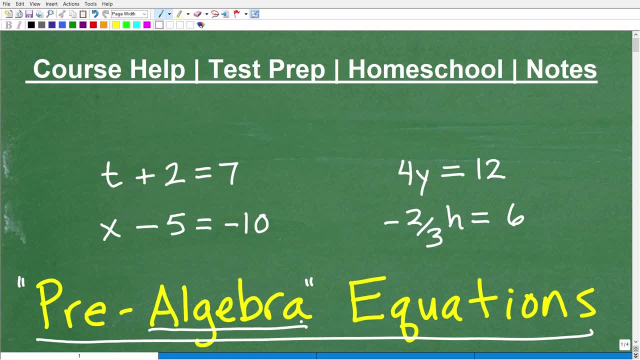 my math help program in the description of this video. but if you think you are a bad math student, maybe you think you're not good at math, maybe you don't feel like you're getting enough math instruction or you're not connecting to your 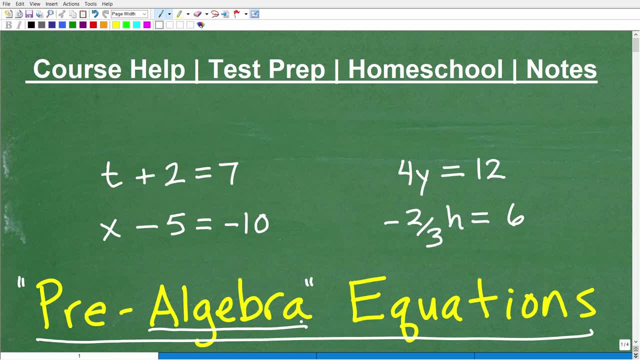 teacher's teaching style. Whatever the case is, whatever difficulty you're having in mathematics, I'm telling you right now there is a solution. Okay, I have yet met a bad math student and I've been teaching math for decades. If you're struggling in math, there's a reason behind. 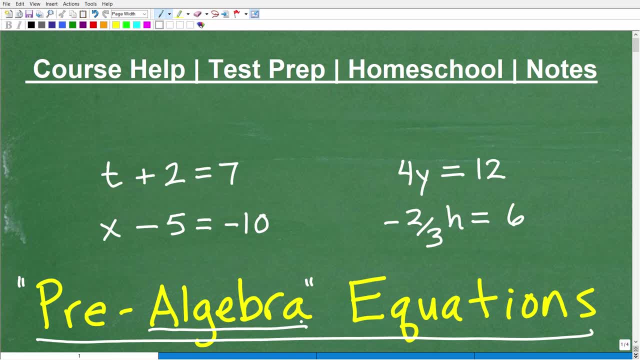 there Okay, and whatever the reason is, it can be solved. but the most important thing you need is two things: One, you need the desire to learn- You've got to be willing to work hard- and two, you need the right instruction, and I like to believe I have that right style of instruction. 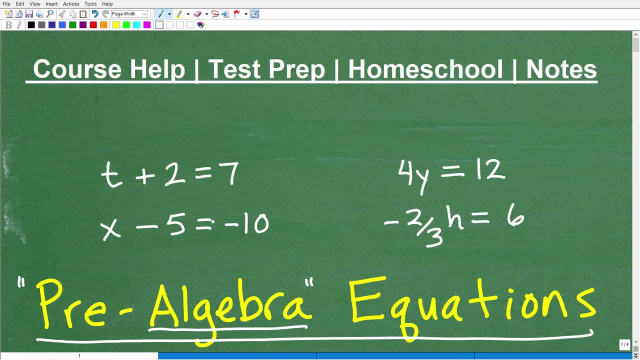 because I like to really explain things in super easy, understandable, bite-sized pieces so anyone and everyone can learn math. So if you're at the middle school, high school or college level, definitely check out my math help program if you're having a tough time in mathematics. 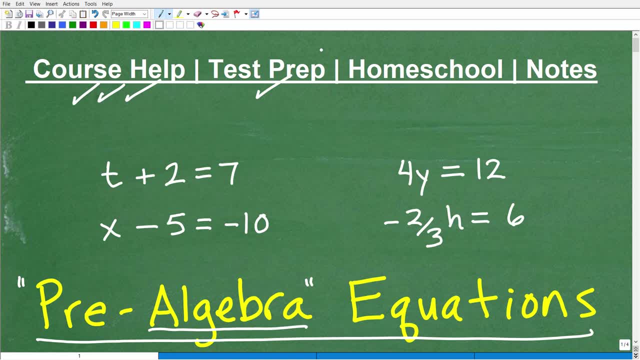 Now, if you're preparing for any kind of test that has a math section on it- I'm talking about things like the GED, SAT, ACT, GRE, GMAT, ASVAB, ACCUPLACER, CLEP exam, maybe a teacher certification exam- I can help you prepare and pass those exams. 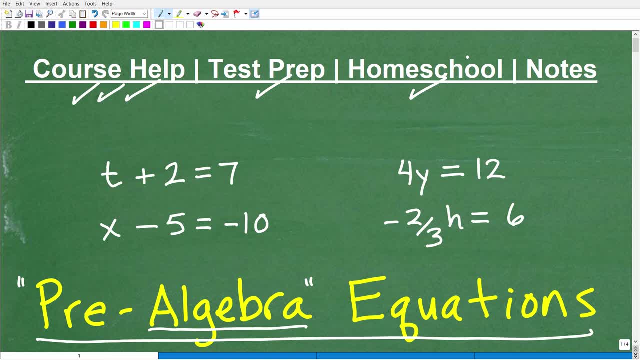 If you homeschool, you definitely got to check out my homeschool math courses. We were just voted number one from a major national publication in homeschooling for middle and high school math. Very proud of that achievement. and if you don't have any math notes: 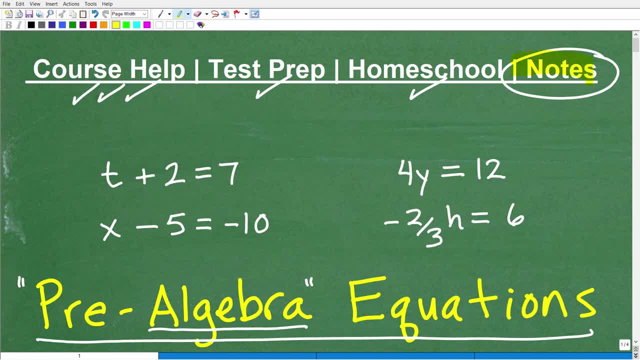 I'm going to leave links to my math notes in the description of this video as well, but I got to tell you right now: if you want excellent grades in mathematics, you need to learn excellent math notes. So start improving your notes and everything will start getting better. 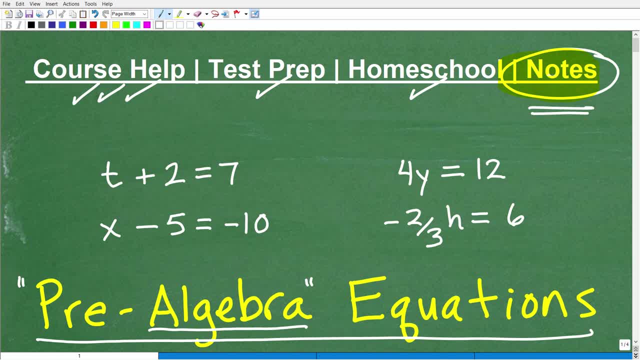 for you. All right, so let's get into these problems. We have four basic equations, and each one of these equations to solve or to get the solution to these equations is going to require one step. Okay, so there's one step. Now the step that we're going to be doing is going to 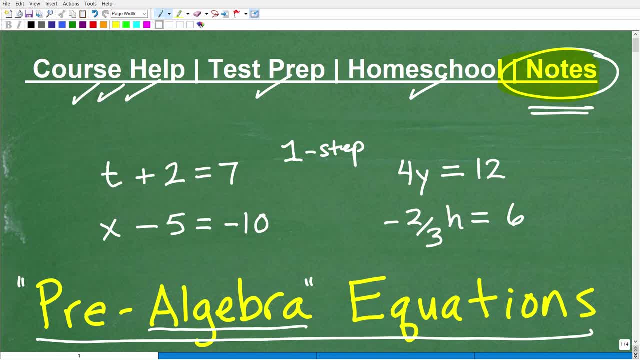 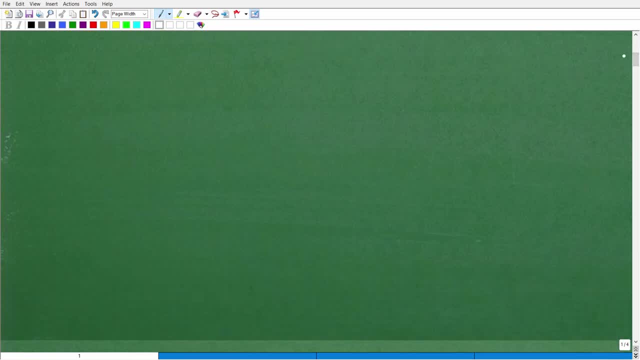 be different for each of these equations, but it's just going to be one step to get the solution. So let's go down here real quick and talk about what you're going to be learning in pre-algebra and algebra one and beyond in terms of solving. 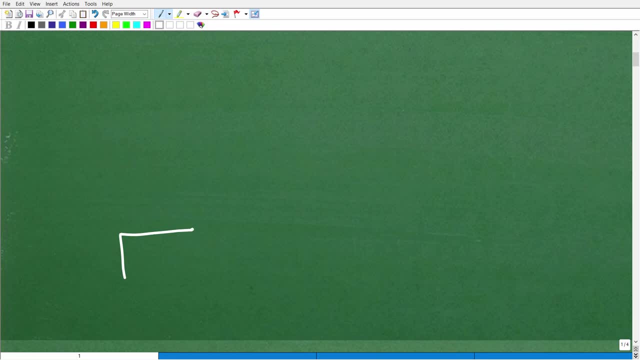 equations. So think of it kind of as like steps, like you're going to be climbing some steps And let me just kind of do it like this. So the first type of equation you're going to be solving, okay, right here, is called a one step equation, Something like this: 2x is equal to eight. 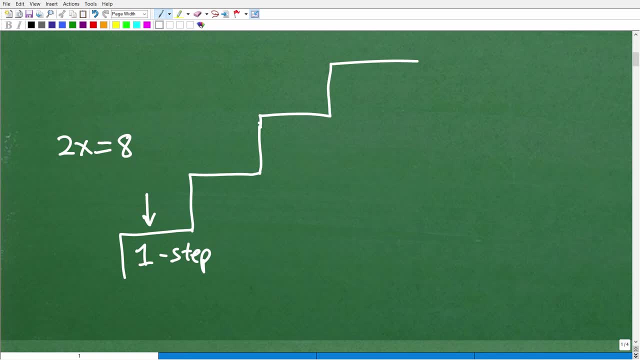 we literally just have to take one step to get the answer. answer So when you're studying like equations and pre-algebra, and you can actually do a little bit of this even in more like middle school math. In fact, you were doing some of this stuff in. 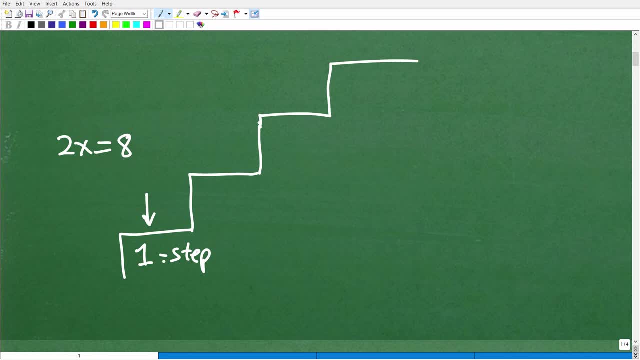 elementary school. you just didn't realize it, But to get the solution to this equation requires literally one step, And that's what we're going to be practicing in this video. Now, once you get these equations down, you move on to what type of equations do you think we're going to be doing? 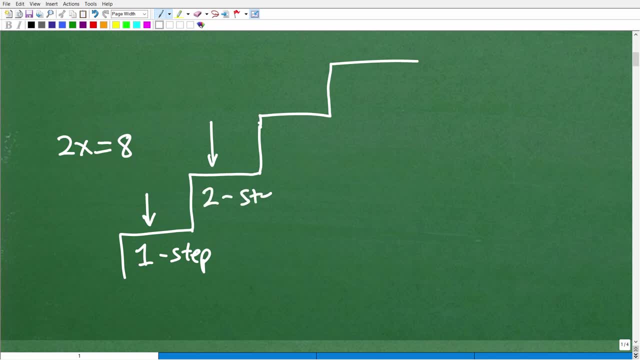 next, If you said two steps, well, I tell you that is very impressive. It shows me that you're paying attention to the video, So that's excellent. So that would be an example of like: say three y minus one is equal to eight. Okay, so to solve this particular equation, you need to take two. 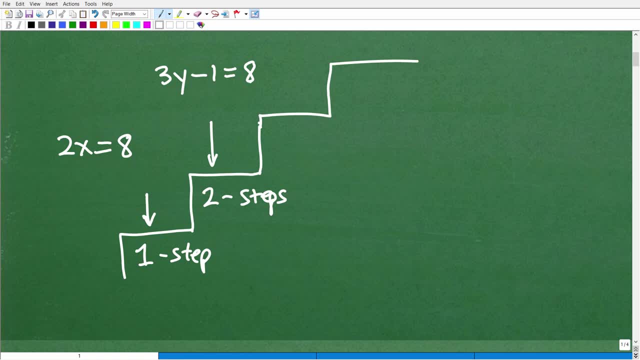 distinct, exact steps. Okay, take one step and then you take another step and you solve these type of equations. So what do you think comes after? Um, two step equations? Now, if you said three step equations, that's a pretty good answer. But 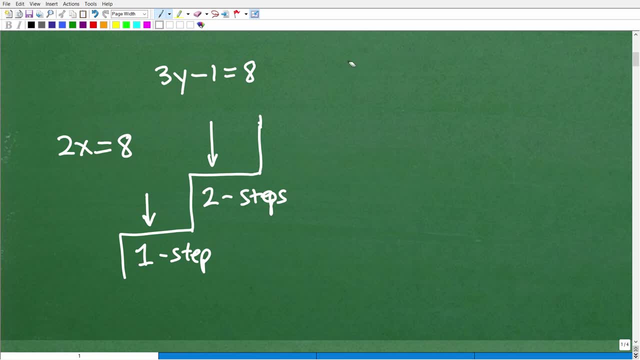 in fact, it's not the way we describe it. Okay, I'm going to go ahead and erase my little stares here. What you really have is something called multi-step- Okay, multi-step equations, And that could be something like this: Let's say, two h minus one is equal to seven h plus two times two. 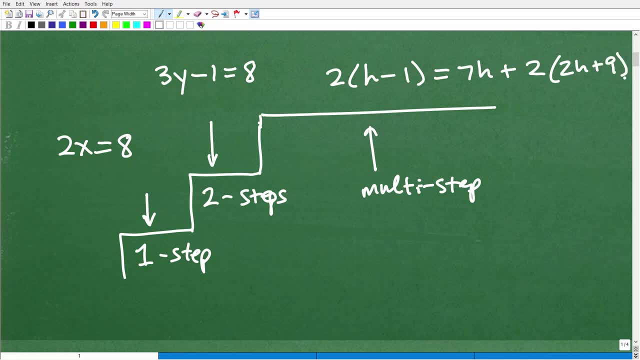 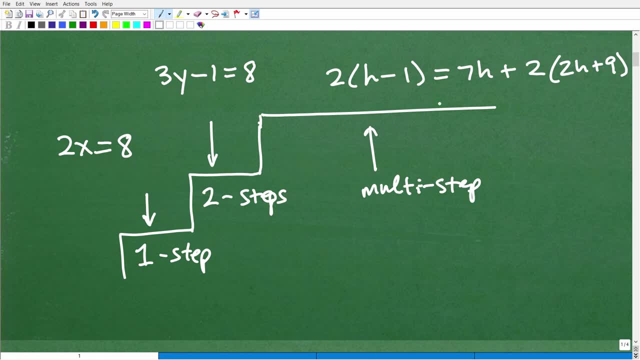 to solve this particular equation you're going to have to take multiple steps, But but the steps you're going to be taking are nothing more than a bunch of one step type of procedures. Okay, so whatever steps we learn here, we're just kind of just doing two of them in this problem And then 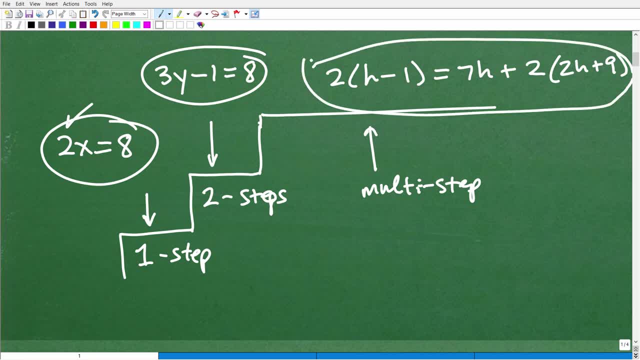 we're just doing a bunch of these same kind of steps in this particular problem. So there is a equations. this is kind of the path they're going to be taking. So the type of equations you're going to be focusing on in this particular video are one-step equations. Of course, this is 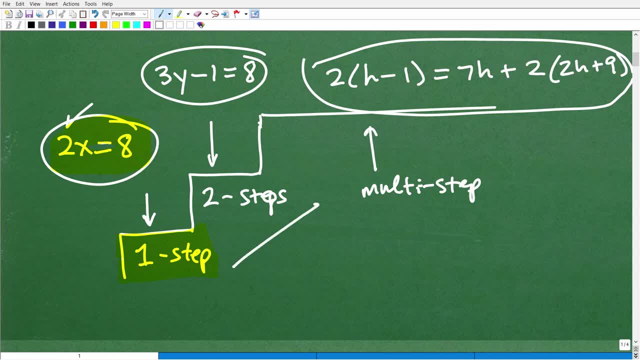 stuff that you really need to master at the pre-algebra level. And then all of this is: you know, you get into like Algebra 1 and, of course, Algebra 2.. Okay, so hopefully that kind of gives a little bit of the context of what we're going to be doing here And we're going to start off. 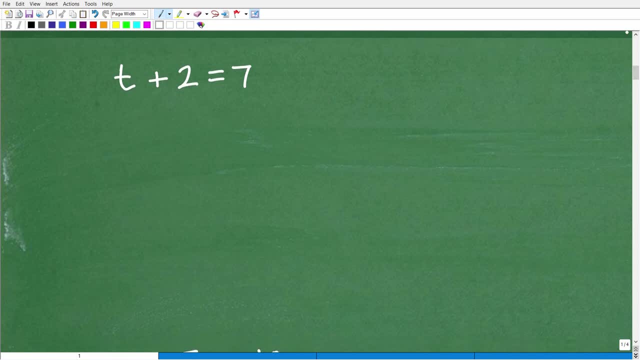 with our first equation right here. Okay, so again, we're talking about one step. And what is this one step? Well, here, I could just show you the step, but I really want to explain this to you, Okay, well, one thing you need to know is that an equation is like a balance scale. Okay, it's like 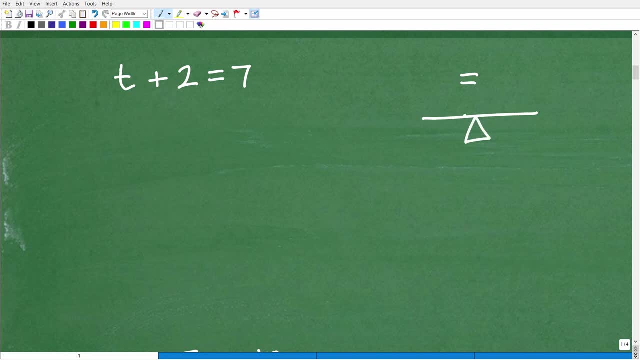 this. There's a little fulcrum there: a teeter-totter, a seesaw, whatever you want to think of This thing always has to stay in balance. So, whatever you want to think of this thing always has to stay in balance. So, whatever you want to think of. 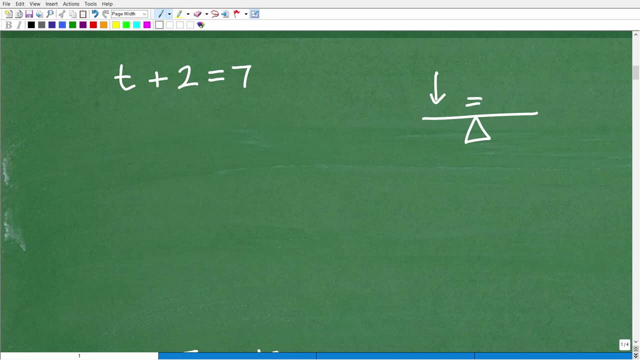 whatever you do to one side of the equation, okay, whatever step you take, you have to take the exact same step on the other side of the equation. You can take whatever step you want to do. You can add, subtract, multiply, divide, As long as you do it equally to both sides. you can never disrupt. 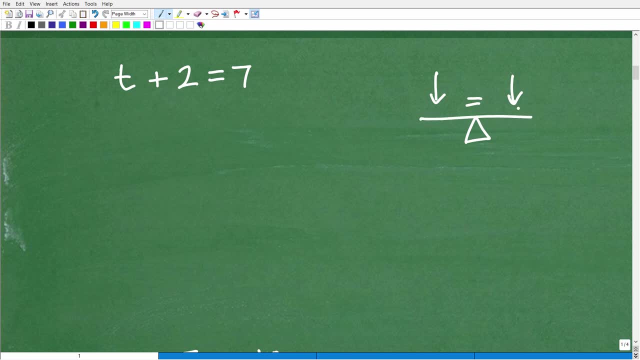 the balance of the equation. Okay, so that's number one. Number two: what is the goal of this equation, or any equation? Well, it's to figure out what the variable is equal to. So here we have the figure out: what t is equal to, What number is t equal to, And that particular number, if we plug. 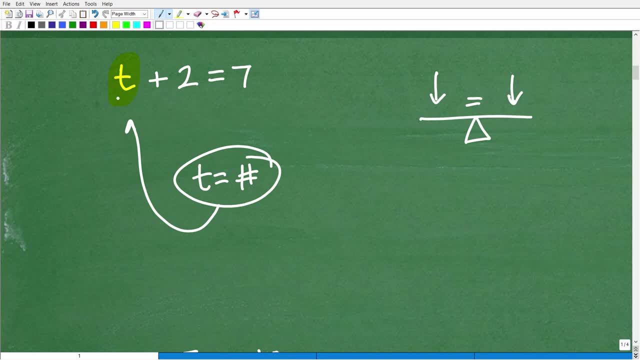 it into the equation. this is a solution if, in fact, it balances this thing out. Okay, so these are just big picture concepts that you need to know and keep in mind when you're solving any equation. All right, now, as we get going here, I'm going to show you how to do this in a second 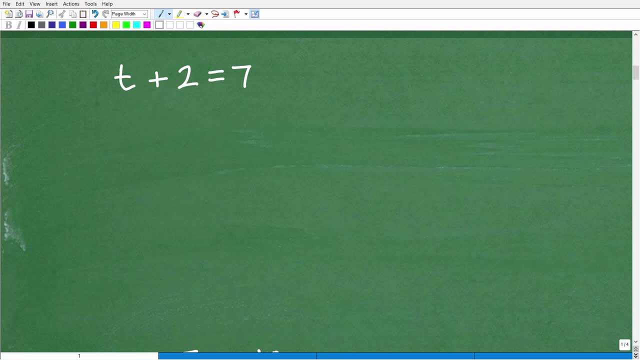 I want to really encourage you to follow my format to solve these equations. It's probably the most typical format, but there are a couple. well, there's like another way of writing showing your work. Don't do it this other way, okay, And 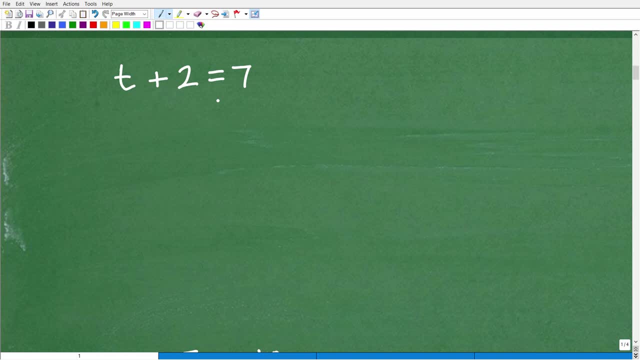 this other way. I'm not even going to mention it, Just do it my way. It's probably the most common way, anyways, in terms of how you write this stuff out. Okay, so let's get going here. So we have: t plus 2 is equal to 7.. So I want t by itself. Remember t by itself. that's the solution. 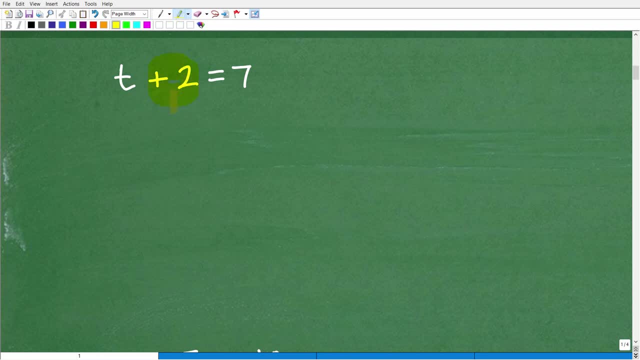 Again, I have t plus 2.. I got this plus 2 over here. I'm like you know, I don't want this thing next to the t, I just want t by itself. So how about we just subtract 2 from this 2? Okay so. 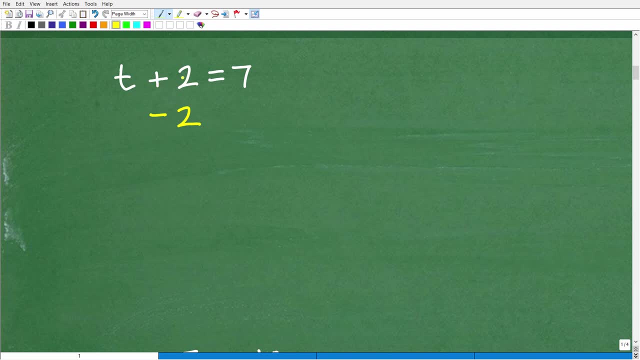 if I have a positive 2 and I subtract a 2 from it, that's 0. It basically makes that go away. But remember the rule in algebra: Whatever you do to one side of an equation, you have to do the exact same thing to the other side. So in this case, 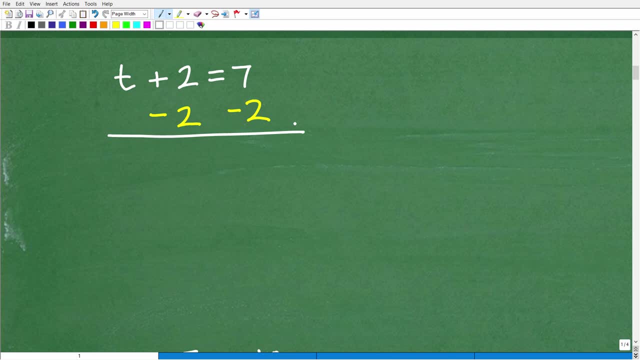 we're going to subtract 2 from both sides of the equation, okay, And then what you're going to do, it's kind of add down in a column manner, So t plus nothing is t okay by itself, And then positive 2 minus 2 is 0. So all we have over here is t, Okay. t plus nothing is just t. This goes. 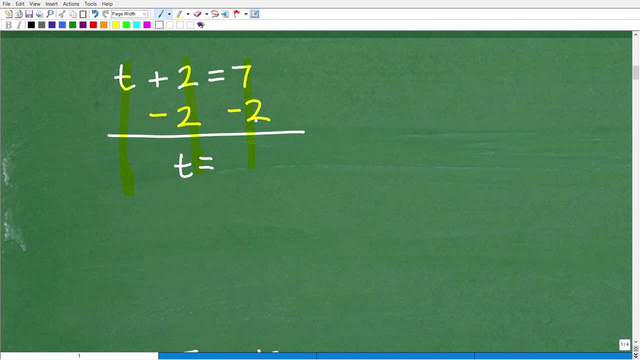 away. We don't need to write that 0. And then 7 minus 2 is, of course, 5.. Now, most of you probably saw that 5 was the solution here, But what we're really practicing here is stressing. 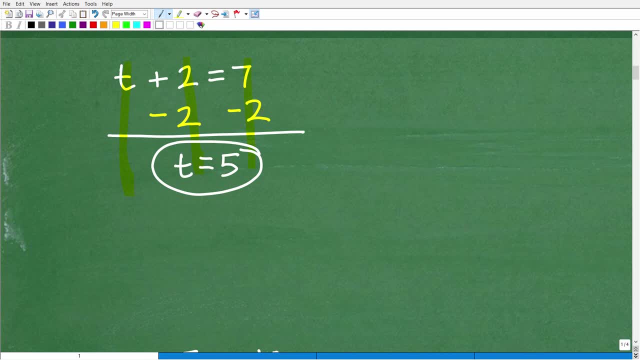 the principles, the mechanics, the big concepts that you need to truly, really understand to solve any equation. And we're starting off with these basic equations, But again I want to emphasize: you know, hey, whatever you do to one side, you got to do to the other side, And then 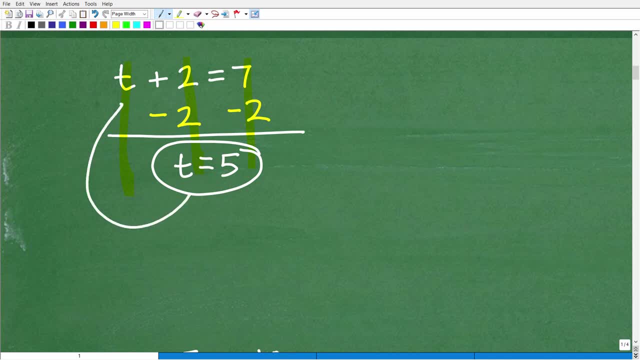 this value. right here is the solution. If, in fact, if I plug it back into this, if I replace a 5 with this t right there, let's kind of check the solution to make sure it's accurate. So if I have t plus 2 is equal to 7, I'm going to replace this t with this 5.. Okay, so let's do that. 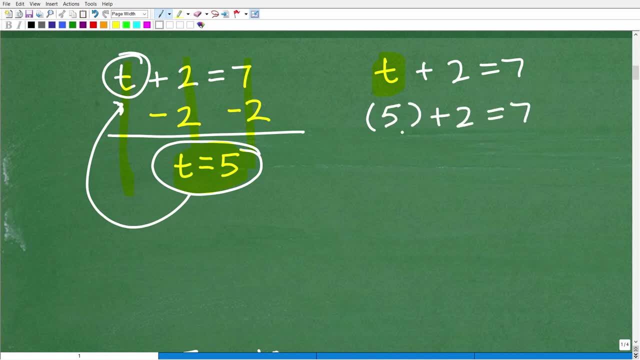 now, And then I'm going to check my work. All right, so 5 plus 2 is 7, and 7 is equal to 7.. That's a true statement. So because when I replace this 5, okay with the t, and I got the left-hand. 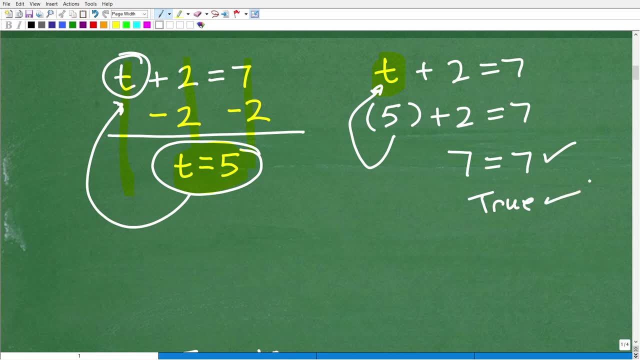 side equal to the right-hand side, which of course is true. that is, in fact a valid solution to that equation. Okay, so remember, you know the mechanics is easy. You could say: oh plus 2,, just subtract. 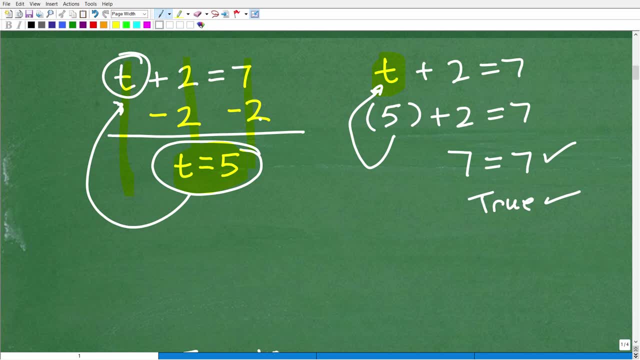 2 from both sides, get the answer. Yes, you know, I think obviously I could make this like a one minute long video. I could just do this, these problems, real quick. But I'm really trying to stress here is, for those of you who are studying basic equations is to really kind of understand. 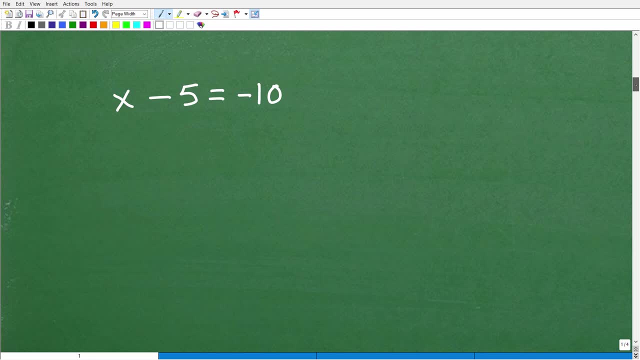 the basics, the fundamentals. Okay, all right, let's move on Now. we'll pick up the pace just a bit. And now, if you think you could do this problem, okay. this is very similar to the previous problem. it's going to require one step, And what do you think that first, 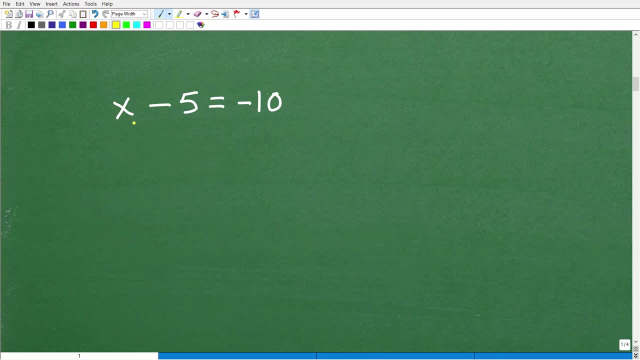 step is going to be Okay. well, if you said: well, we got x minus 5, we want x by itself, how about we get rid of this negative 5 by adding a 5 over here? Okay, let me write that. 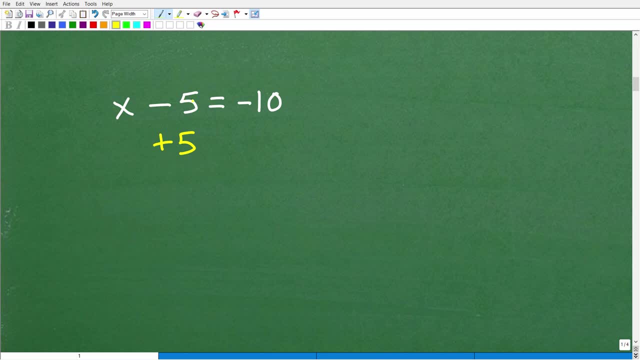 a little bit better. So negative 5 plus 5 is 0. That gets this x all by itself on the left-hand side, So I can add a 5 over here. Okay, remember, I want to keep this format. then you're going to be adding down. 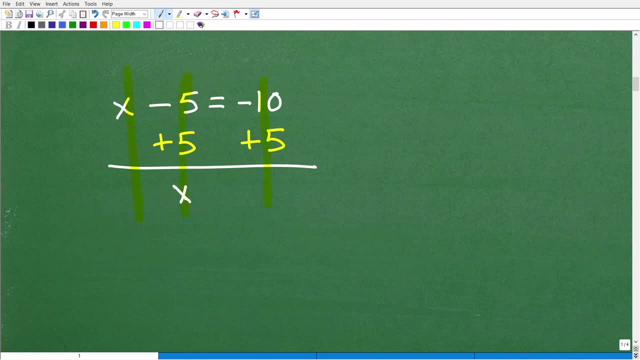 In a column manner. So x plus nothing is x, or write that right there. Negative 5 plus 5 is 0. We don't need to write that. 0 just kind of vanishes. And now I have negative 10 plus 5 is negative 5.. That is the solution. Now you could see here that you need to understand. 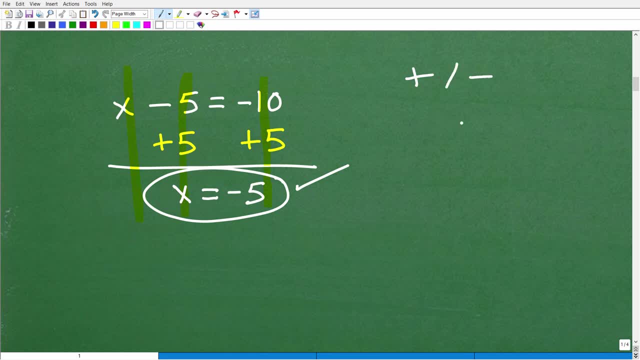 positive and negative number rules. So this is definitely a big deal at the pre algebra level, in like at the eighth grade math level. Make sure you understand how to add, subtract, multiply and divide positive and negative numbers. Okay, so hopefully this didn't trip you up, But if you were kind of confused about 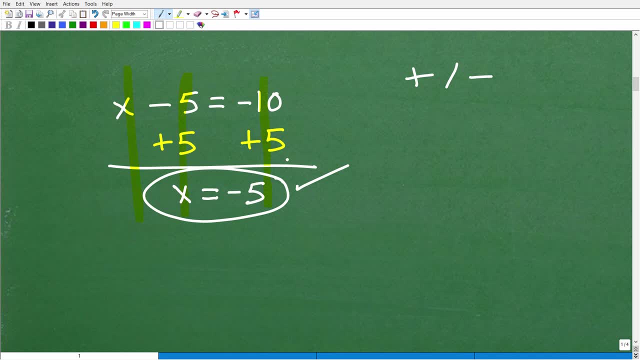 this. well then, make a mental note and go back and review. Let me give you a couple of suggestions. One: I have tons of videos on my YouTube channel- my pre algebra playlist- on this more basic level of algebra and positive negative numbers, etc. Or I teach this super. 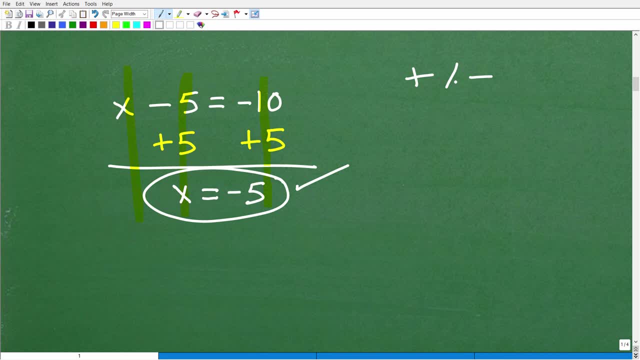 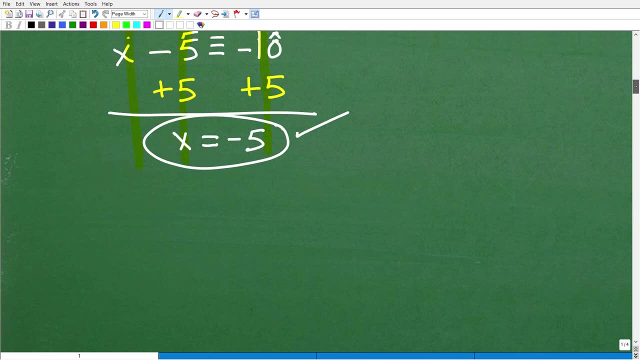 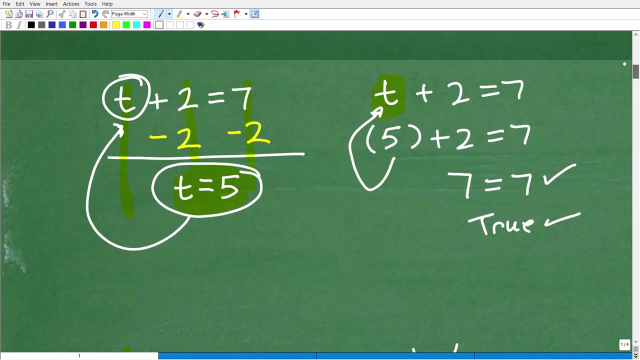 thoroughly in my pre algebra course as well. Okay, so let's move on To our next problem. All right again, just see here. all we're doing is taking one step, the first. the one step is just adding five to both sides. we got the solution here we're. 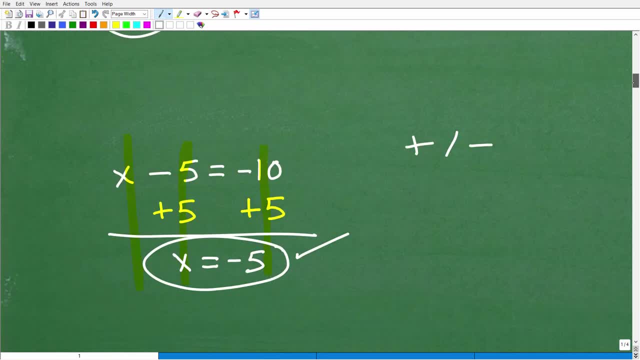 subtracting from both sides. we got the solution, So let's move on down here and continue on with these one steps. So what is this equation? Well, it's four y's equal to 12.. But what does this mean? in algebra, this four in front of the y means multiplication. Okay, so let's. 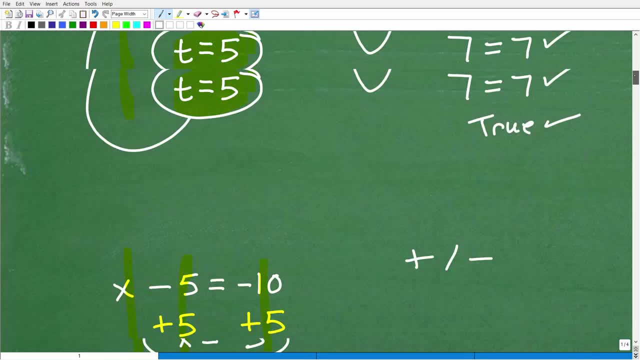 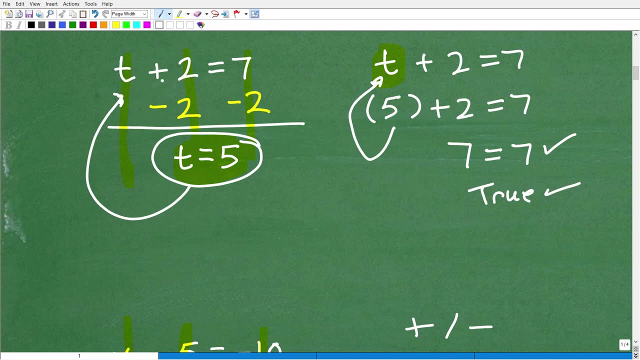 go back over here. I've kind of missed a point And I want to kind of bring this in Now. notice, in our equation right here, when we have t plus two, okay, t plus two is equal to seven. we ended up. but the step that we took involves subtraction, Okay. so when we 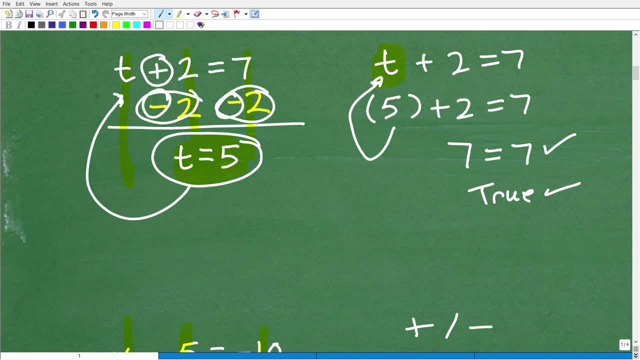 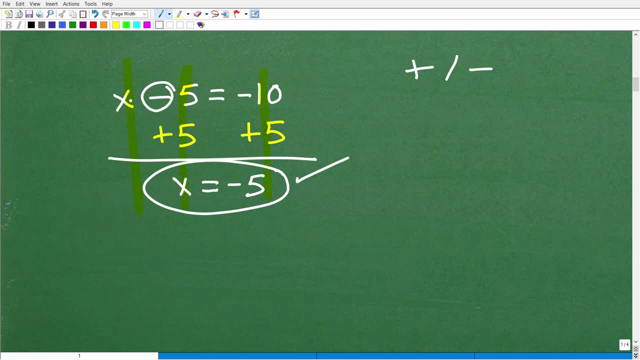 saw an addition, we ended up using subtraction to get to that solution. Okay, so that's what we call it: inverse operation. Now notice over here: When we had subtraction x minus five, we ended up using addition to get to the solution. 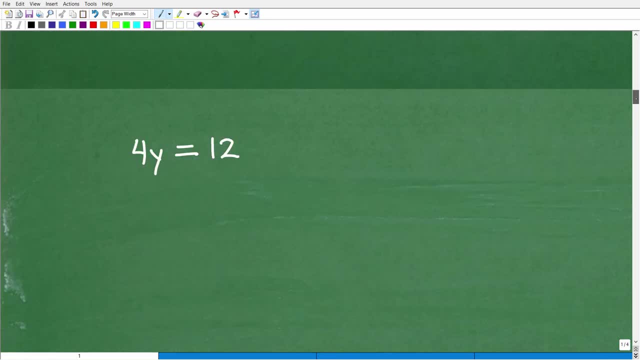 Alright, so keep that in mind, because this is very, very important. And over here we have four times y. this means when you have a four or a number in front of a variable, this means multiplication. Okay, so what is going to be the inverse of multiplication? 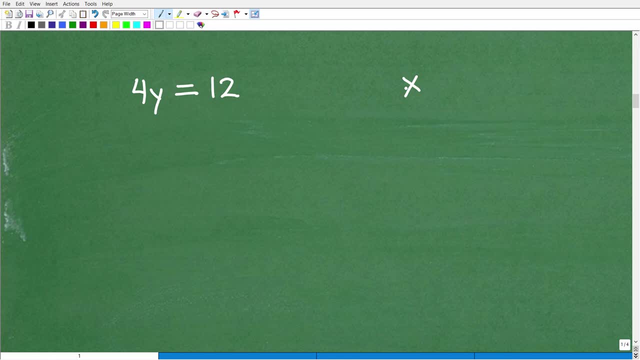 What do you think? the inverse, What's the opposite? Operation, mathematical operation that you would associate with multiplication. Well, hopefully, you said, is a division. you would be correct. So, just like addition, it's inverses subtraction with subtraction, its inverse is addition for multiplication, its inverse. 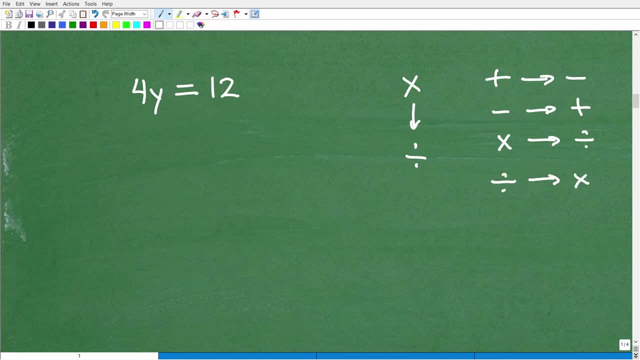 is division and with division, its inverse is multiplication. Okay, so this is another thing that you want to kind of remember when you're solving these basic equations. So we're dealing with the multiplication here, we want to undo this. just get y by itself. so i know, now that you know that this is multiplication, you're thinking: 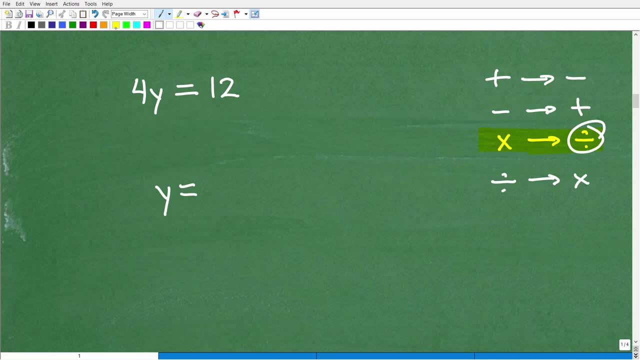 division. all right, like okay, what's the one step we can do here? hopefully, he said: oh, i could just divide this side of this equation by four, because four divided by four is one. okay, one y. that's what i want. now. we don't write uh, variables like one y, like this, we just write it like this y. this means. 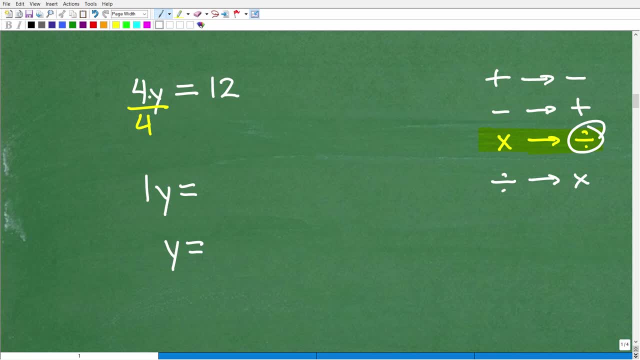 one y. so i got to this y by dividing whatever this number is, i just divide it by itself. on this side of the equation, i get one y or y, and that's exactly what i want. so let me go ahead and put that here. but again, let's remember the rule. okay, whatever you do to one side of the equation, you 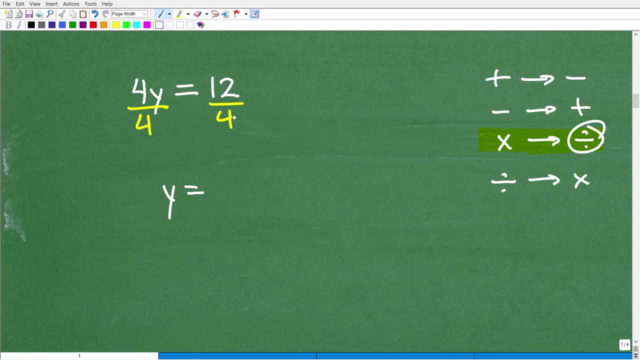 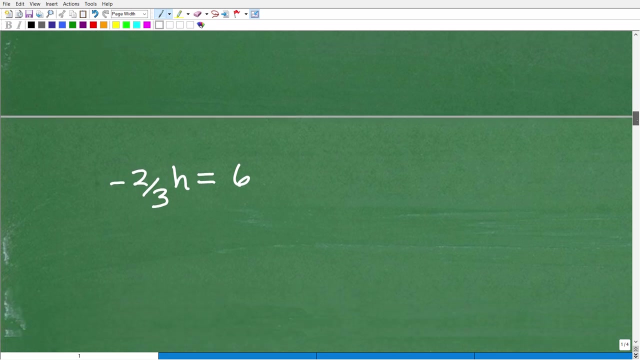 got to do the exact same thing to the other side. so we have 12 divided by four, which, of course, is three. there's our one step and there is our solution. okay, so hopefully you're getting pretty comfortable, you this, and i saved the- uh, the most challenging one, or the one that tends to confuse students- uh, the. 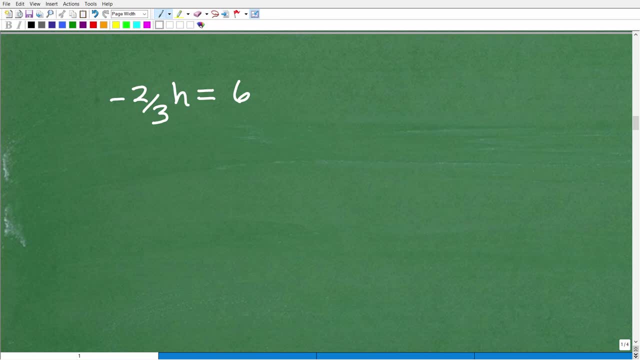 most. so let's take a look at this problem. so what does this mean? well, i have negative two-thirds times h. now i'm going to write this a little bit differently here. negative two over three times h. uh, it's really. i'm just writing this this way, it's just to make this a little bit easier for you to. 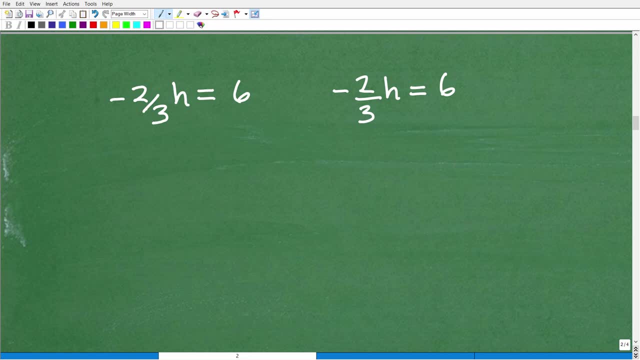 see that the way you write these fractions right here this way, with a little slash or with a little uh uh kind of complete horizontal bar, it doesn't make a difference, both are perfectly fine. but let's take a look at this. okay, so we have negative two-thirds times h. so you might be thinking 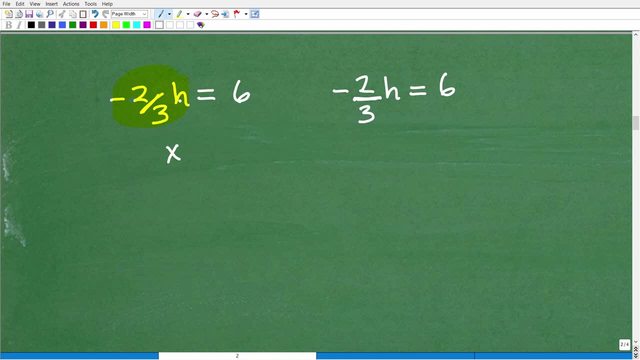 to yourself: well, this is multiplication, because this is this number times this. so maybe we need to divide both sides of the equation by this number. okay, whatever that number in front of that variable. so maybe we need to do this: this negative uh divide both sides equation by negative two-thirds. and if you uh were thinking: 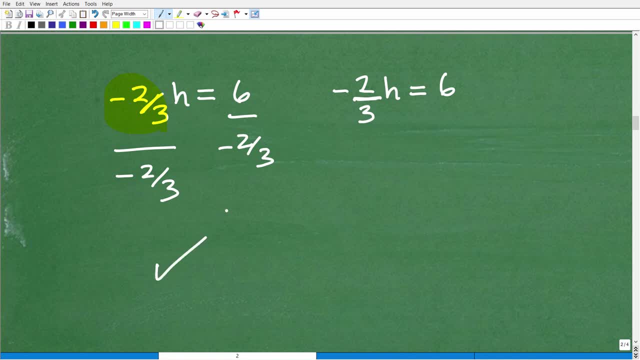 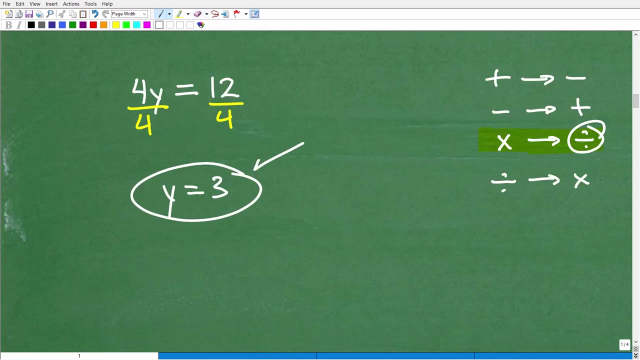 in these terms to solve this equation. you would be correct. okay, so that's good, that's very good. matter of fact, this will get you the right answer, but i want you to uh kind of uh key in on something else here. let's go back to this previous problem and remember this problem here involved. 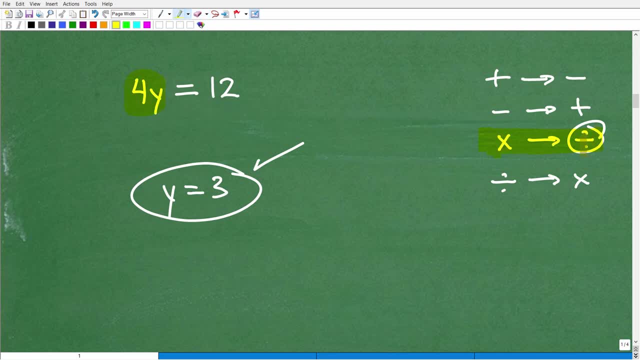 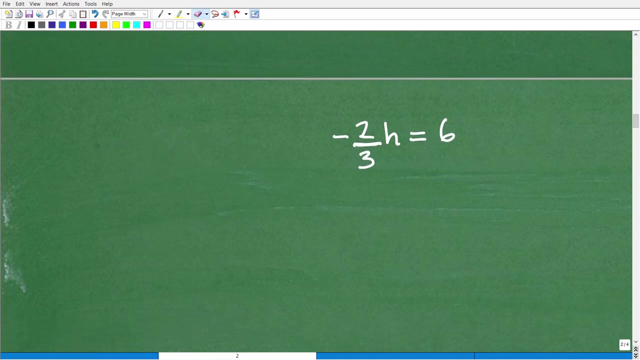 multiplication. so we say, okay, multiplication is division. now, in this next problem we're going to be doing, really, what we got is a division problem, so we can use multiplication to do this. so let me show you how we want to kind of think about this and let me use this version of the problem, okay. 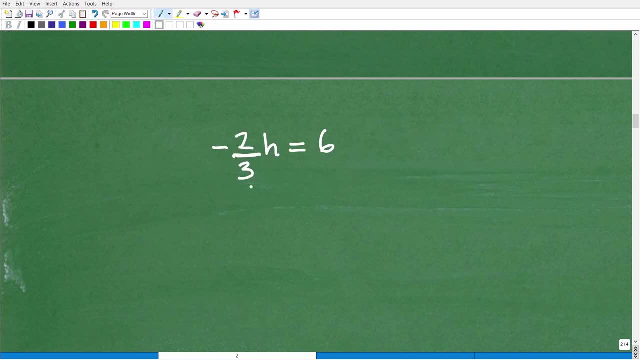 so we have negative, uh, two divided by three. okay, so what's the goal to solve this? well, we want to get h by itself. so this right here is division. okay, there is multiplication going on, but i want you to kind of think of it as division problem. so we want to use multiplication to get to the solution. it's the easiest way to remember. 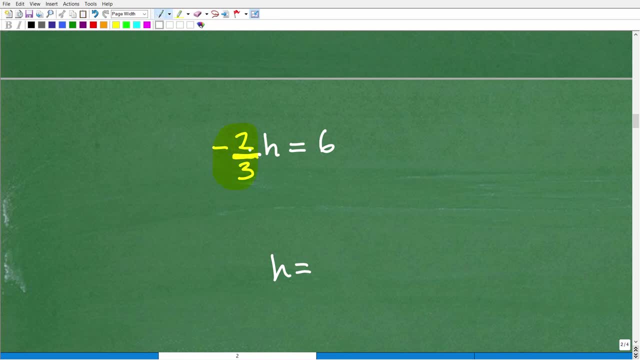 how to do this. so let's take a look at what's going on here. so we have this fraction negative two divided by three, or negative two-thirds. if i multiply this side over here, what i'm going to do is i'm going to flip this fraction, so that's going to be three over two, and i'm also going to keep 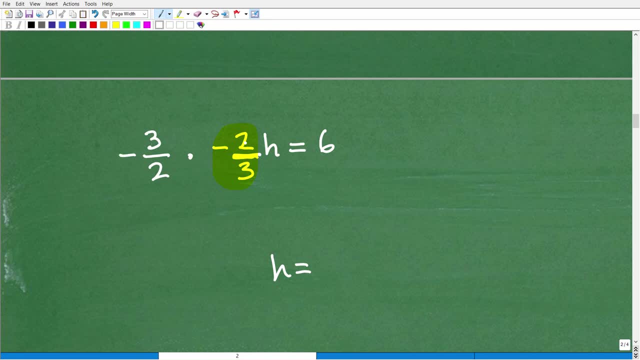 the sign negative three over two and i'm going to multiply by this negative two-thirds. okay, anytime you multiply a fraction by, it's what we call. it's reciprocal. if you flip it upside down, you're always going to get one, a negative times a negative is a positive and then three times two. 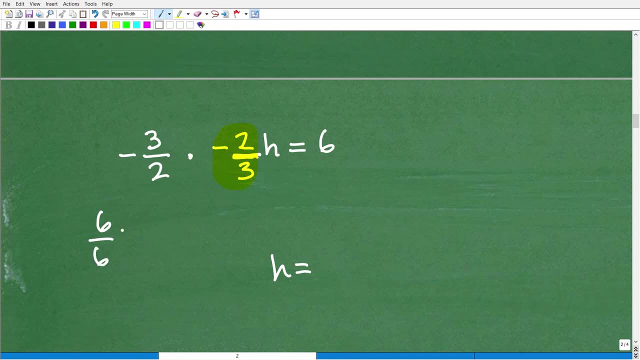 is six over two times three is six. so six over six is one. we're going to get one h, and that's what i want. i want an h all by itself. so over here, the way to handle problems when you have a fraction coefficient, in other words, a fraction in front of 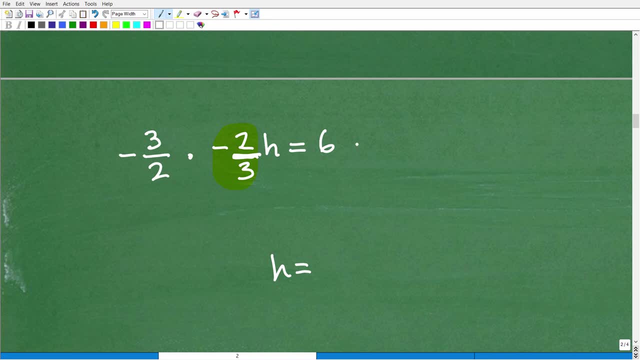 a variable is just to flip that fraction upside down and multiply both sides of the equation by that reciprocal, ie that fraction that we flipped upside down, and you need to keep that sign as well. so if it's negative, keep the negative in that reciprocal. in other words, if this is negative, 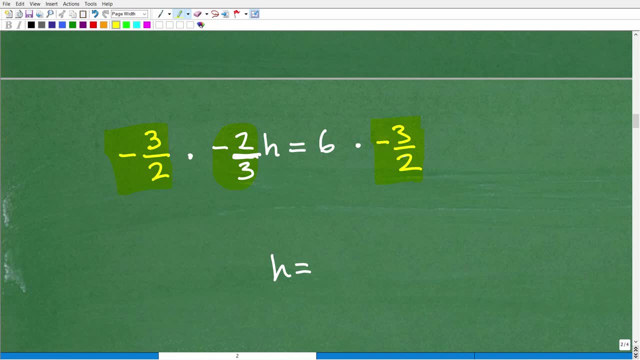 you have to multiply both sides equation by that negative fraction. if it's positive, you're going to multiply by the positive version of that, all right? so let's go ahead and do this math. so six times negative, three over two, so that's six over one, right? so six times negative, three over one times two, which of course is two. 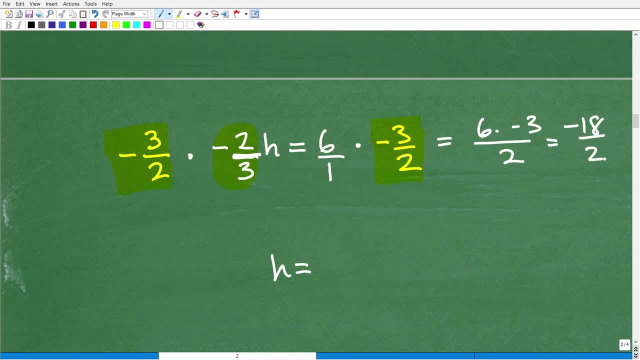 six times negative. three is negative: 18 negative. 18 divided by two is negative nine. okay, so this is negative nine again. you need to know your positive negative numbers and how to work with fractions to do these basic one-step equations. and i'm actually going to be posting a video, very, very. 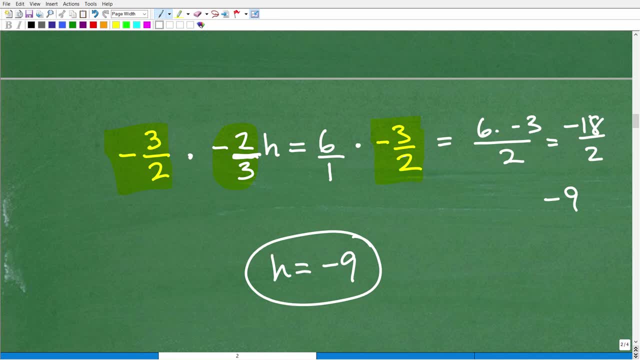 shortly about the math you need to know to be successful in pre-algebra- okay. so again we're taking pre-algebra. we're looking at pre-algebra type of equations which you need to know for algebra one. but to be successful in pre-algebra you need to know all that stuff in middle school. 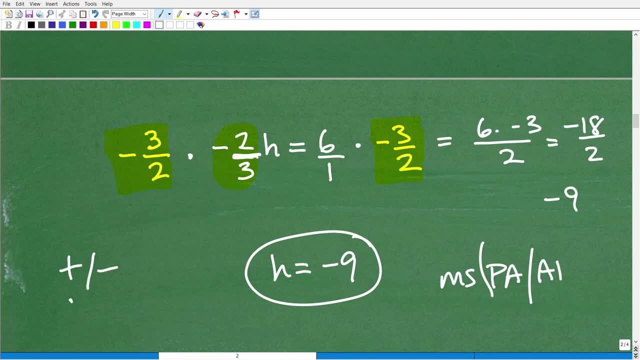 math, which would include the basics of positive, negative, numbers, fractions and some additional things as well. so whatever basic skill you know you are not quite understanding, just make a mental note of it and go back and review. but if you understood all of this, okay right now, and you're. 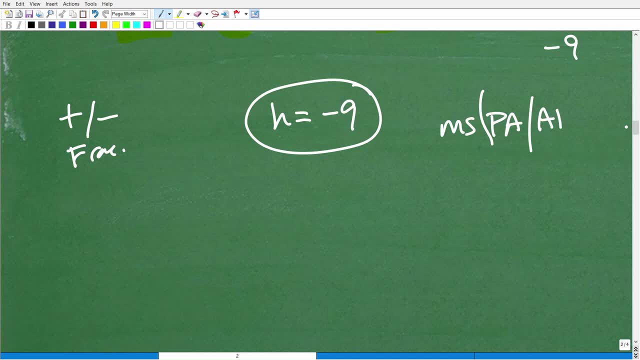 like, yeah, i just wanted to check myself and see if i got this, not only got the answers right, but really truly understood, uh, the steps you need to take and the concepts behind it. then i must go ahead and give you a good old 1984. uh, mohawk, i gotta throw some colors in, because you know these. 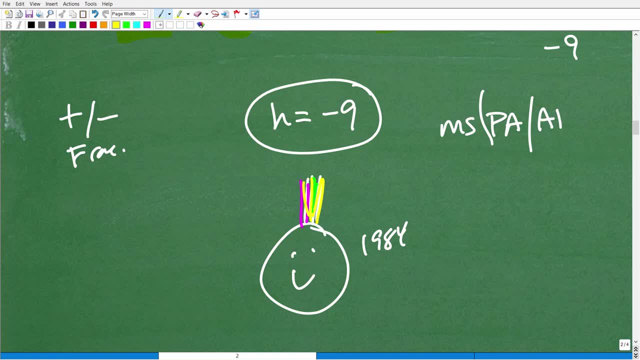 mohawks were pretty impressive back in the day i didn't wear one, okay, but i did have a lot of friends who wore one and we always thought that was pretty cool. but let me go ahead and throw in an a plus. nice job, okay. so remember.